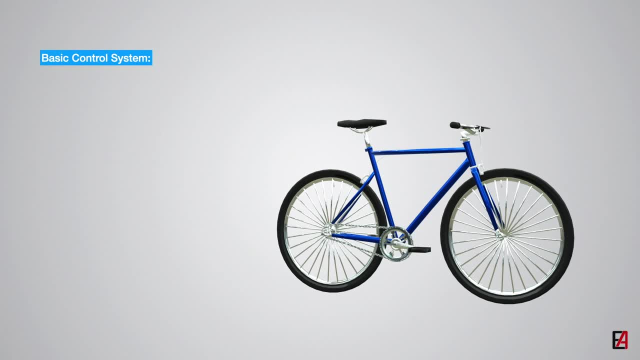 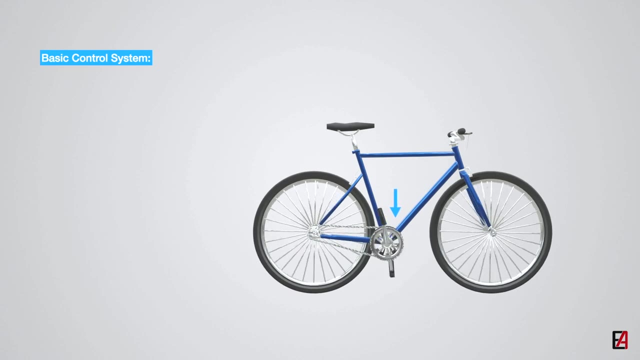 let's take the example of a bicycle handlebar. The direction of the bicycle's front wheels is the controlled output, and the position of the handlebar is the input. Similarly, if the objective is to control the speed of the bicycle, then the amount of pressure on the 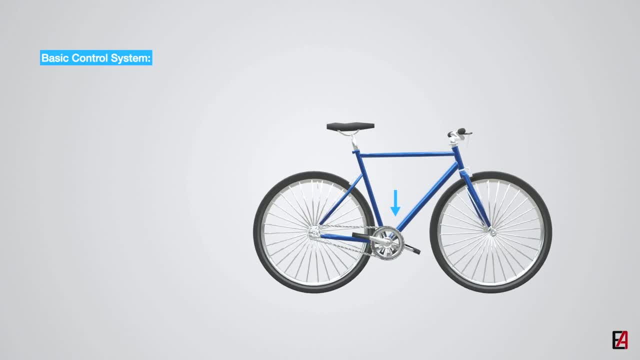 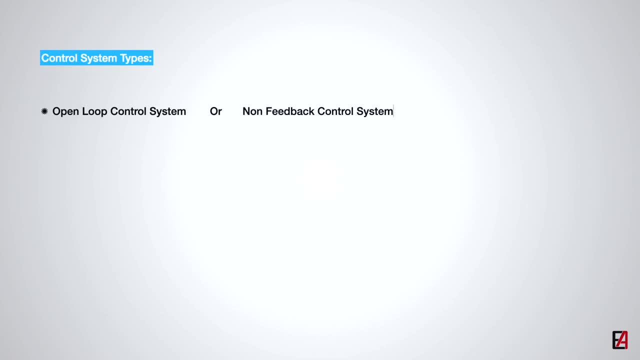 pedals is the input variable and speed is the controlled variable. The two different types of control systems are open loop control system or non-feedback control system, and the closed loop control system or feedback control system. Let's see about the open loop control system first. 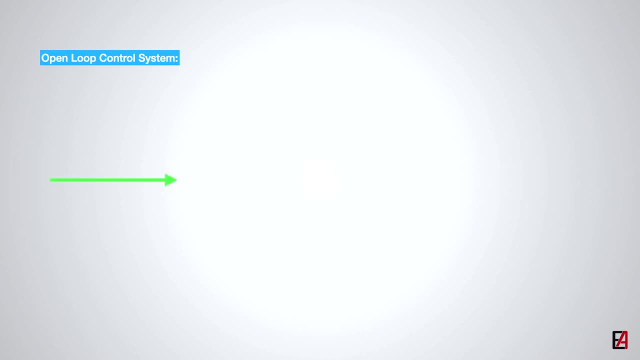 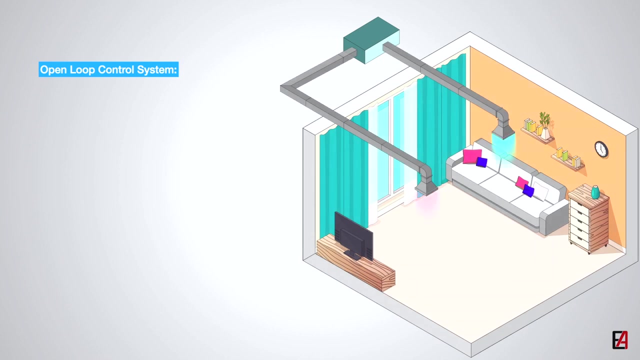 The block diagram here represents the open loop control system, non-feedback control system. An input signal or command is applied to the controller, whose output acts as the actuating signal that regulates the control process and drives the controlled variable to the desired value. To understand this, let's take a living room which is conditioned by a fan curl unit. 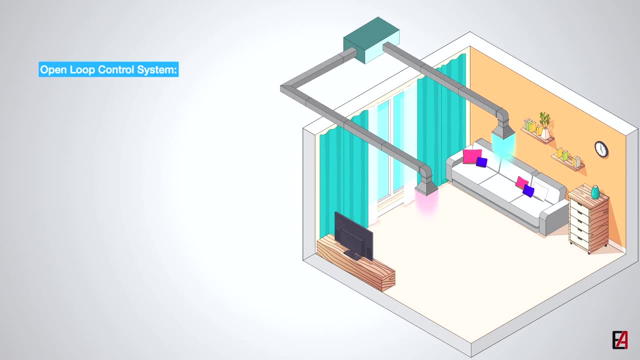 Consider this: FCU works on a time-based temperature control sequence where the chilled water control valve is opened and closed based on defined time interval to maintain the room temperature In this defined time schedule is the input to the controller. The actuating signal is the output to open or close the control valve. actuator. 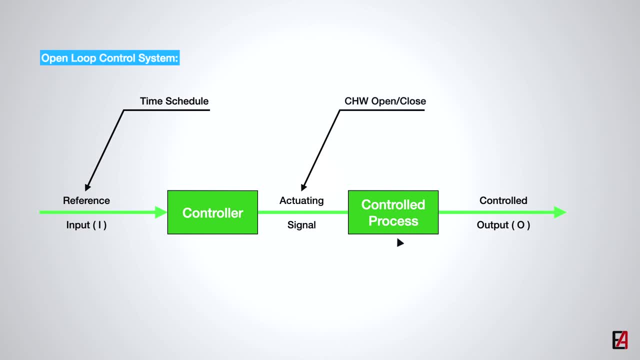 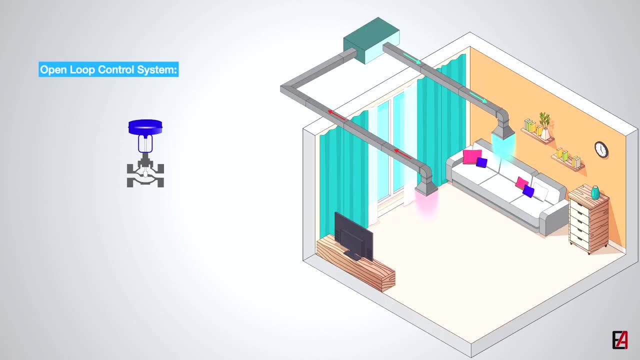 The control process in this example is the room temperature control and the controlled output is the amount of chilled water that is being fed to the cooling coil. Let's assume The control valve is set to fully open for 30 minutes continuously and to fully close. 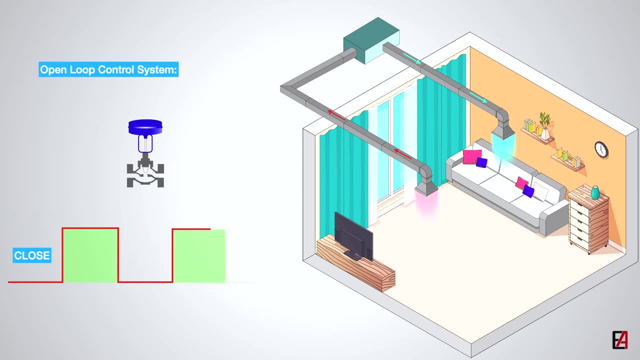 for the next 30 minutes. So the control valve operating cycle is 30 minutes open, 30 minutes close, and so on. During the control valve open cycle, the room temperature will be below the desired temperature, and during the control valve close cycle, room temperature will be above the desired. 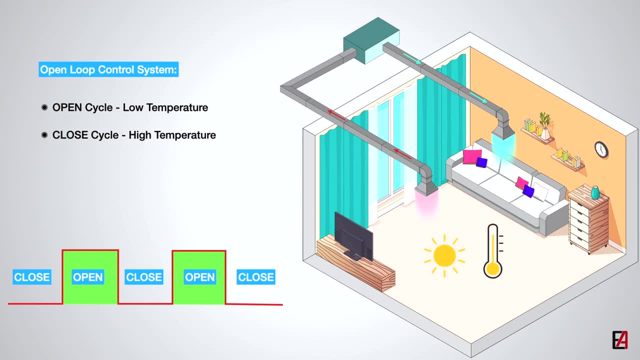 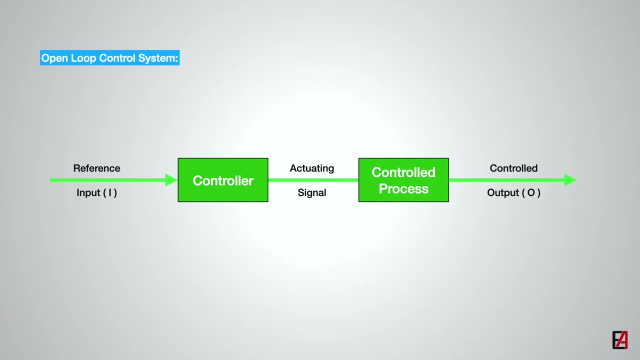 temperature. Thus, it is impossible to calculate the amount of time required to keep the control valve open or close to achieve the desired temperature. due to external interferences such as outside temperature, varying chilled water temperature, etc. It is clear that the desired room temperature cannot be achieved with this type of control. 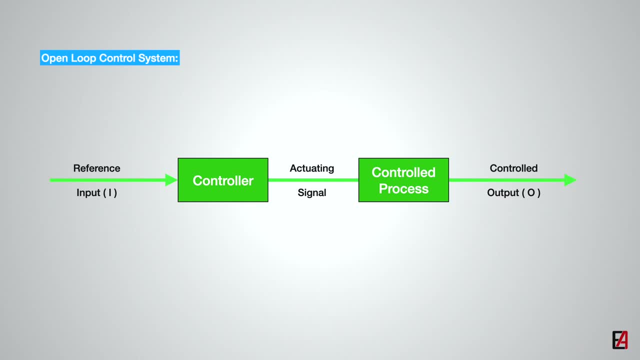 system due to inaccuracy in adapting to external interferences and the unavailability of any feedback signal to the control system to compare with the desired space temperature. So let's see how this works. Another classic example of this open loop control system is a washing machine. 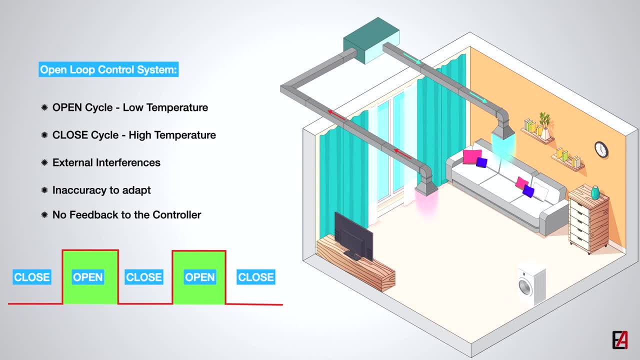 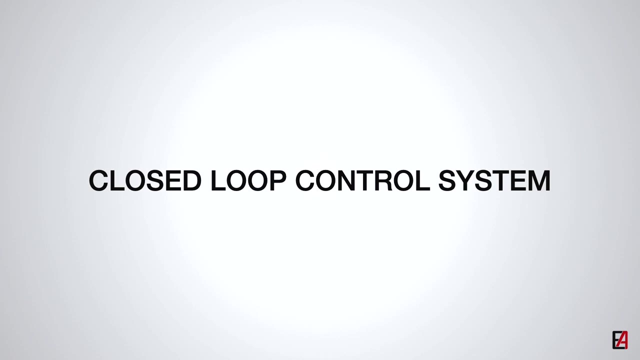 The washing machine operation is entirely depending on the amount of time set by the operator. It is obvious that the clothes may be or may not be cleaned thoroughly. thus there is no feedback to the washing machine about the cleanliness of the clothes. Closed loop control system. What is missing in the open loop control system? 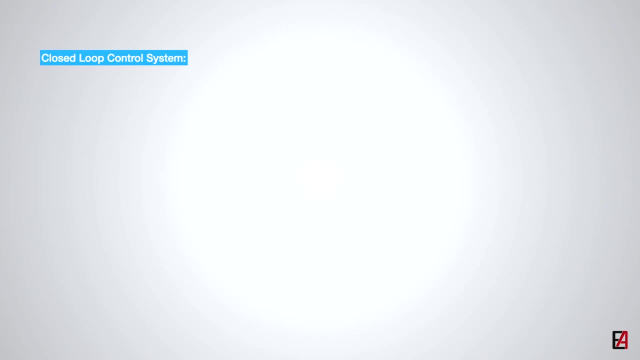 for more accurate and adaptable control is a link of feedback from the output of the system to the input of the controller. In order to obtain more accurate control, the control process must be fed back and compared with the reference input. Then the controller will decide how much activating signal is required to achieve the desired. 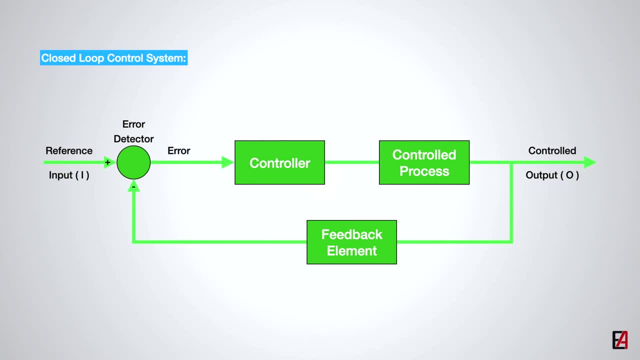 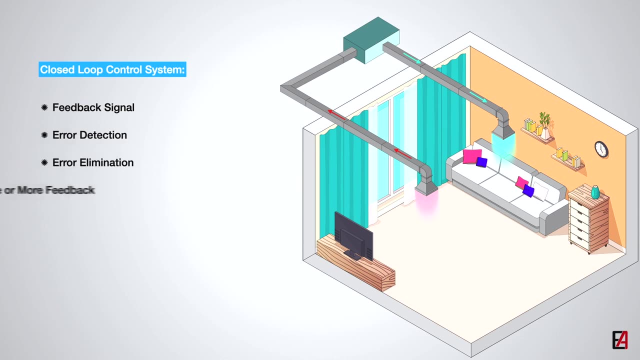 output. The controller will actuate the signal till the error becomes negligible. A control system with one or more feedback is called the closed loop control system or feedback control system. Let's go through the same example. The control system is a closed loop control system. 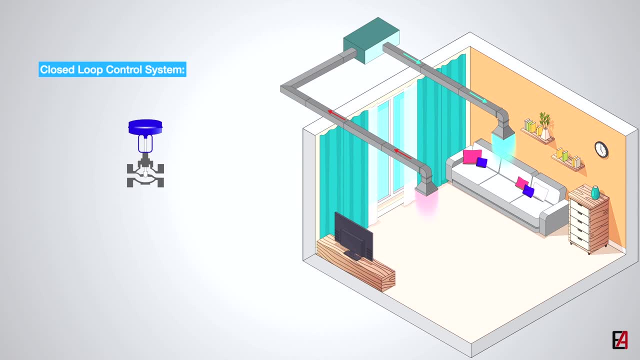 The control system is a closed loop control system. A room temperature sensor, precious to the controller, is provided as a feedback to the controller to calculate the error between the desired temperature and the actual room temperature. Now the controller can decide how much is the chilled water control valve to be opened. 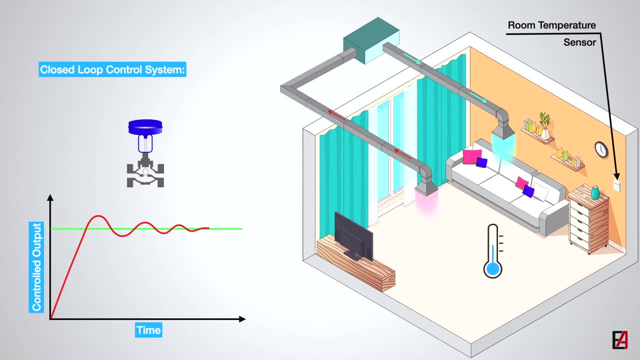 in order to maintain the desired room temperature. The controller will actuate the control valve to eliminate the error, as the controller gets a real time control. For example, if the controller is not operating, the controller can then design. the actual controller gets a real-time feedback of the room temperature. 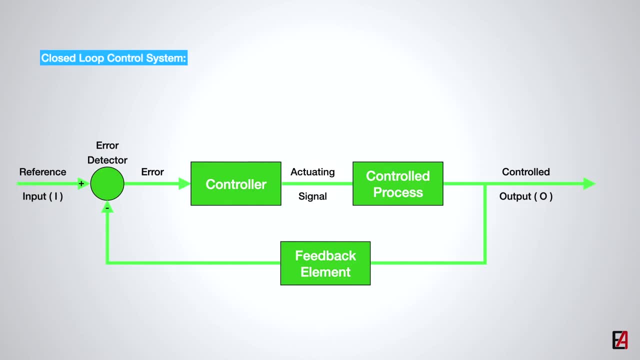 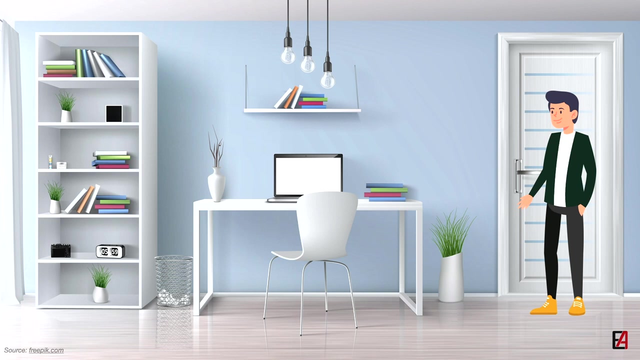 Accurate and stable control can be achieved with this closed-loop control system. Human beings are probably the most complex and sophisticated feedback system, with many inputs and outputs. Let's consider our objective is to reach for a book on a shelf. As we reach our hands towards the shelf to get the book, the brain signals a hand to.